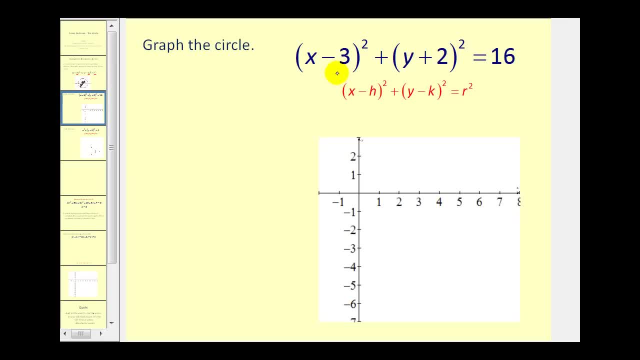 Since this circle is in standard form, we should be able to identify the center and also the radius. Now notice it has to be in the form of x minus h and y minus k in order to find the x and y coordinate of the center. So in this case, the x coordinate of the center would be positive three, and the y coordinate would be negative two, because if it had to be in the form of y minus, it would be y minus a negative two. But a quick easy way to remember the coordinates for the center is, it's always the opposite sign of what you see. If you see minus three, it's going to be positive three. If you see plus two, it's going to be negative two. So this would be the center of the circle, and then r squared is equal to sixteen. If we take the principal square root of both sides, the radius would have length four units. So what that tells us is, if we plot the center at three negative two, the circle consists all of the points that are four units from this point. So what I like to do is go up four units, that point would be on the circle. 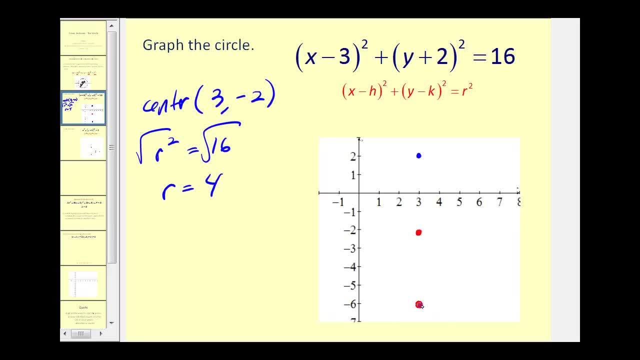 Go down four units from the center, right four units from the center, and left four units from the center. And then from these four points, try to make a nice circle. 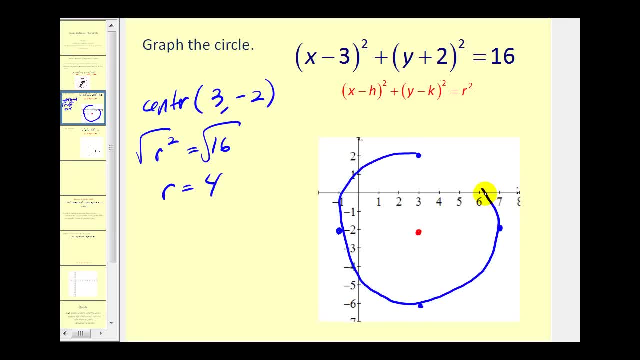 Something like that. So as you can see, when the circle is in the equation as in standard form, it's pretty easy to find enough information to make a nice graph of the circle. Let's go ahead and try one more. 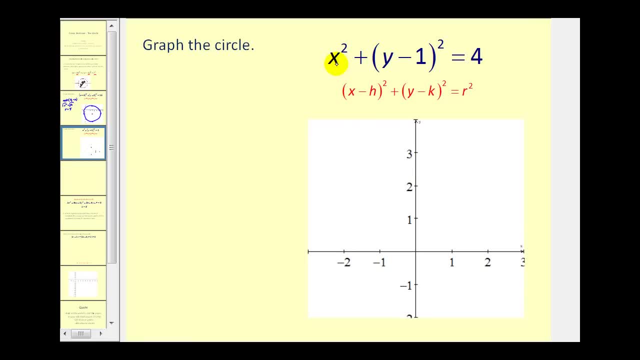 Now even though this form looks like it doesn't match perfectly, we could rewrite x squared as the quantity x minus zero squared, plus the quantity y minus one squared equals four. 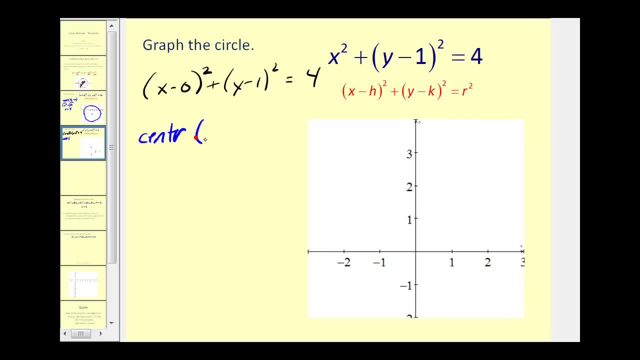 Now the reason that might help is now we can probably determine much more easily that the x coordinate of the center would be zero, and the y coordinate of the center would be positive one. Next, the radius squared is equal to four. So now if we take the square root of both sides, we have r equals two. So we plot the center, zero, one. So the circle consists of all the points that are two units from this point in red. So we'll go up two units, that point would be on the circle. Down two units, that point would be on the circle. Right two units, that would be on the circle. And 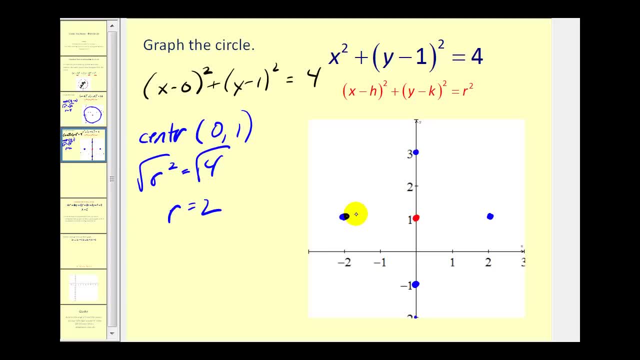 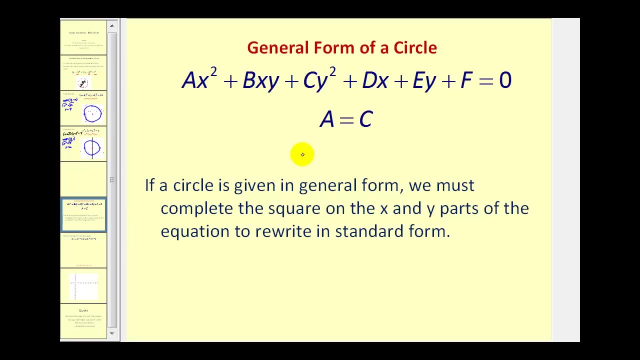 left two units, that would also be on the circle. So now we have to make a circle that passes through these four points. And it would look something like that. Now let's take a look at general form. If we have the general form of a conic section, it'll be a circle if a equals c. Meaning the coefficients of the x squared and the y squared terms must equal each other. 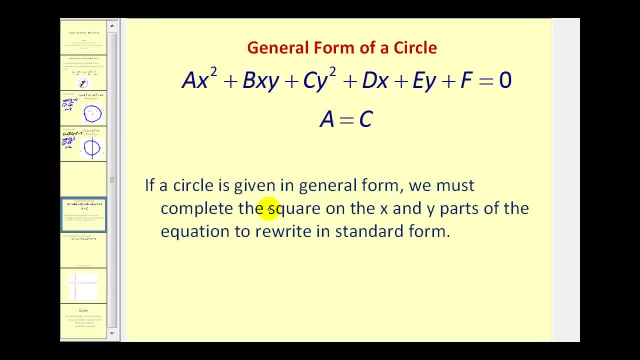 And if that's the case, we have a circle. And what we can do is complete the square on the x and y parts of the equation to rewrite this in standard form and then graph the circle. 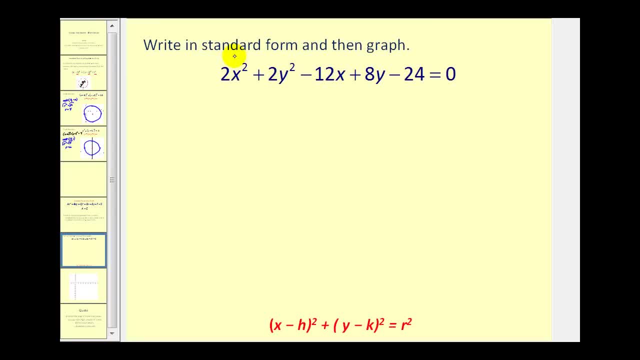 So let's go ahead and give that a try. Notice the coefficient of the x squared term and the y squared term are equal to each other. Therefore, we know it's a circle. 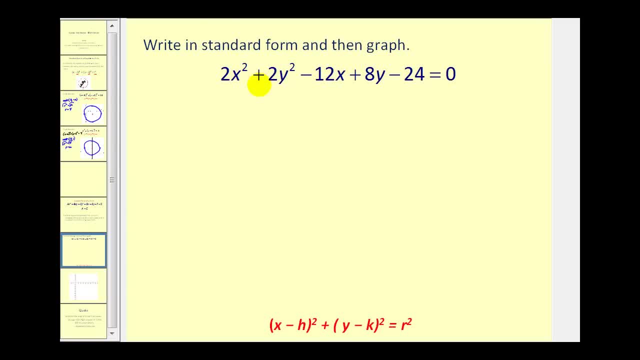 But since we have to complete the square on the x part and the y part, we want these leading coefficients to be one. So what we're going to do is divide every term by two. And of course, if we divide zero by two, we'd still have zero. 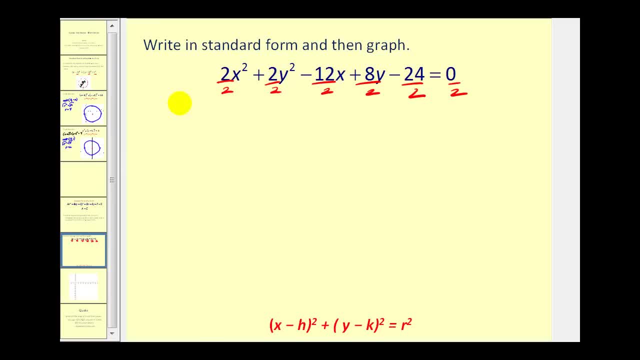 When we rewrite this, we're going to group the x terms and the y terms together. So we're going to have x squared. This will be minus six x. Now since we're going to complete the square on this, I'm going to leave room for the constant term. Plus the y squared term. This will be plus four y. Again, leaving room for the constant term when we complete the square. Next we'd have minus twelve. Or we're going to add twelve to both sides so we have the constant term on the right side. 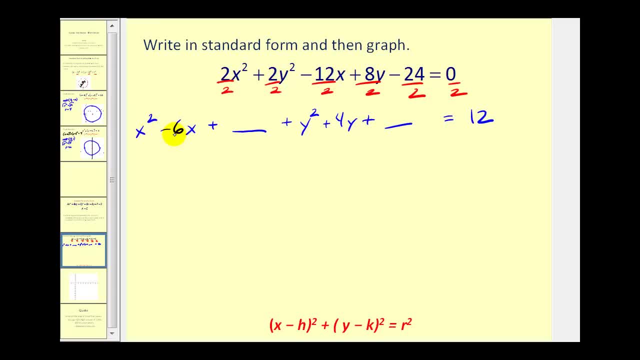 So this would equal positive twelve. Next, remember to complete the square, we take half of this coefficient and then square it. Half of negative six would be negative three. Negative three squared would be nine. So we'll add nine here. And then of course, we have to add nine to the right side as well. Next, we'll take half of positive four. That would be two. And then square it. So we're going to add four here. And add four to the right. Now these should be perfect square trinomials. Let's test it. We want the factors of nine that add to negative six. 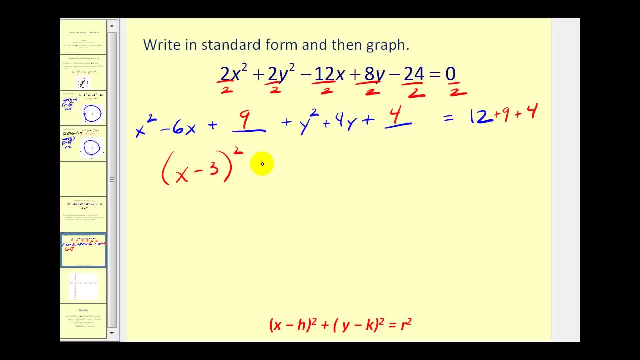 So this factors into the quantity x minus three squared. 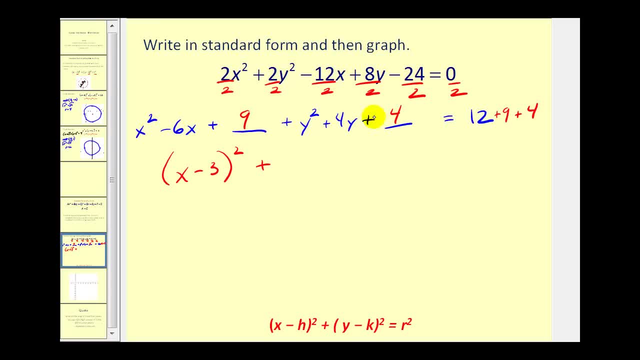 Plus, we want the factors of four that add to four. That would be positive two and positive two. So this would factor into the quantity y plus two squared. 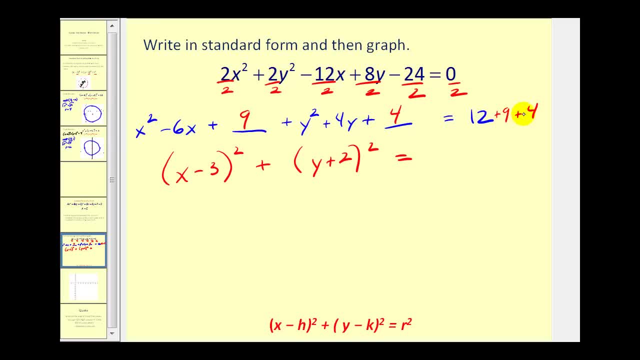 Must equal twelve plus nine. That would be twenty-one plus four. That would be twenty-five. 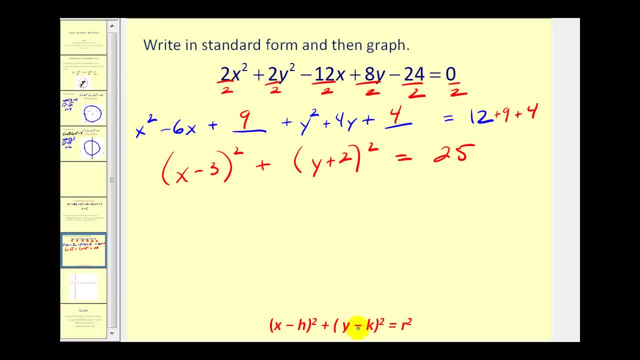 Now the equation is in standard form as we see here below. We should be able to identify the center and the radius. The center would be positive three for the x coordinate. And negative two for the y coordinate. 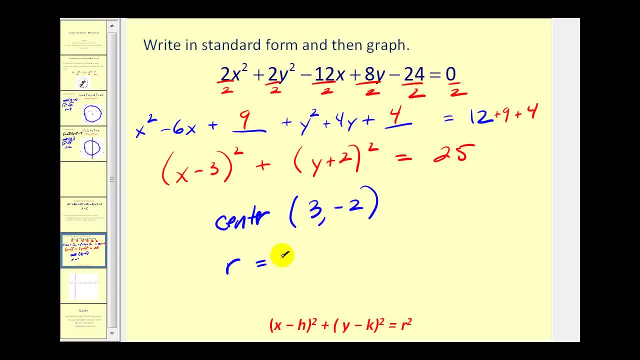 And if this is r squared, then r would equal five. 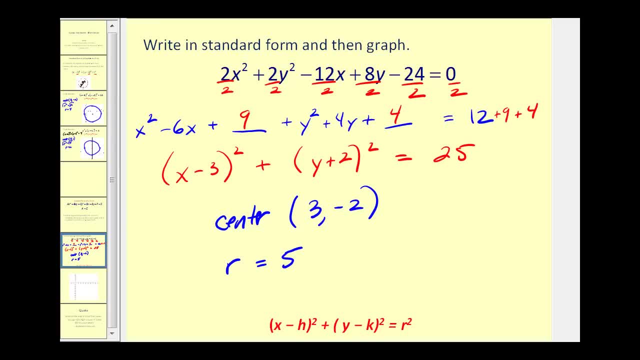 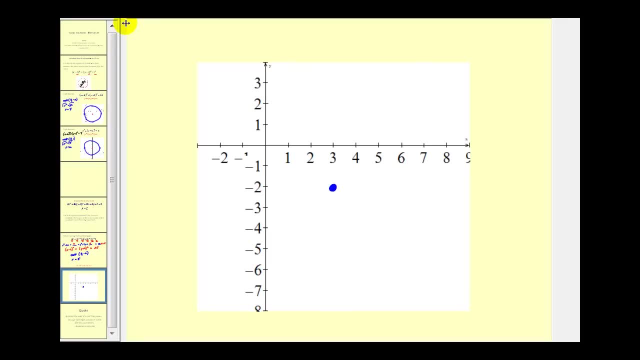 This is all the information we need to make a nice graph. Let's go ahead and graph it on the next screen. The center is three, negative two. And the radius is five. So we'll go up five units. That would be positive three. Down five units would be negative seven. Right five units would be positive eight. And left five units would be negative two. 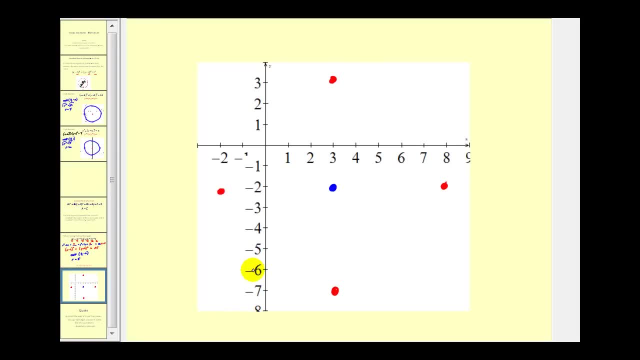 And then we try to make a nice circle passing through these four points. 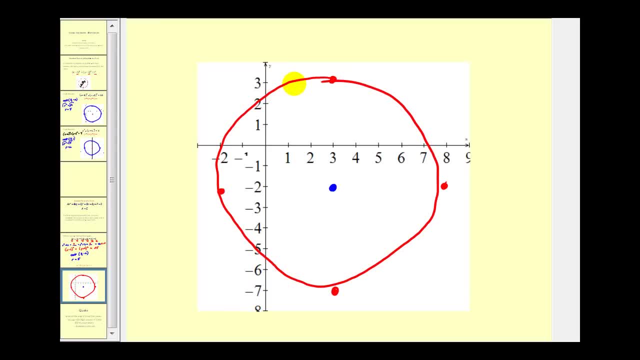 And that's the best I can do. 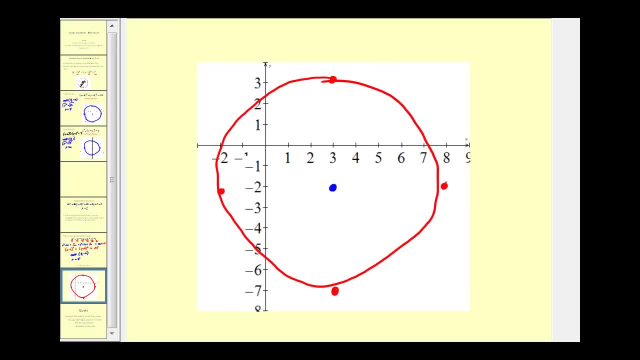 Okay, I hope you found this review helpful. Thank you for watching.